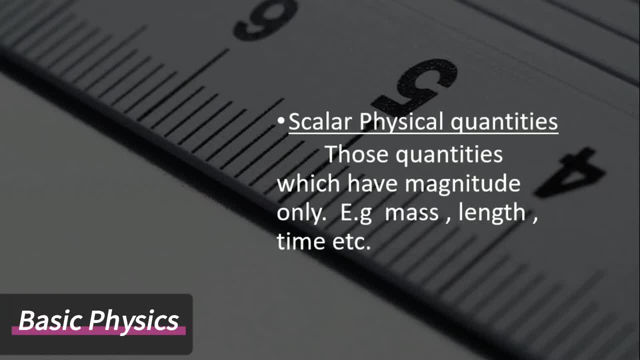 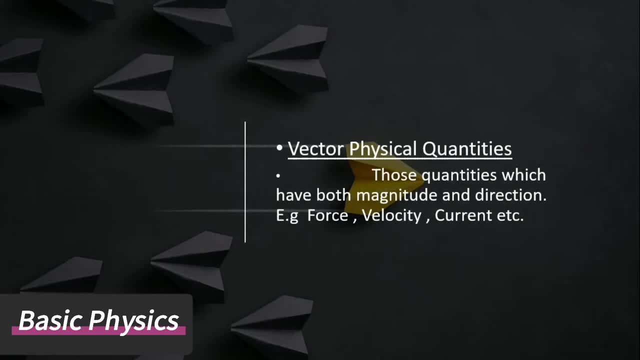 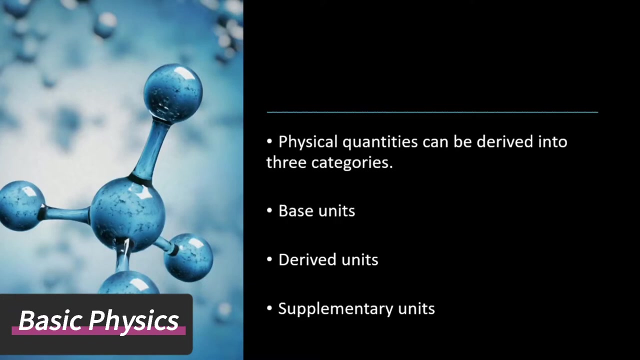 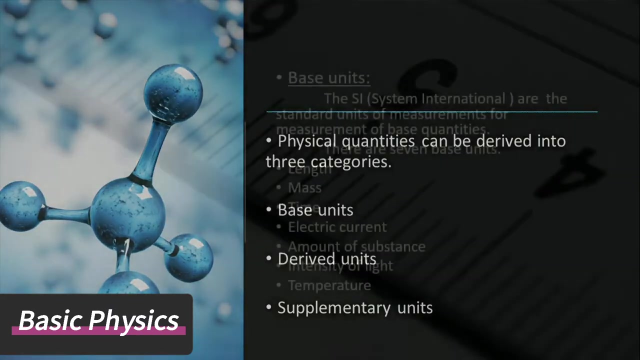 Vector: physical quantities, those quantities which have both magnitude and direction, for example force, velocity, electric current. Physical quantities can be derived into three categories: Base units, Derived units, Supplementary units. The System internation: all are the standard units of measurements for measurements of base quantities. 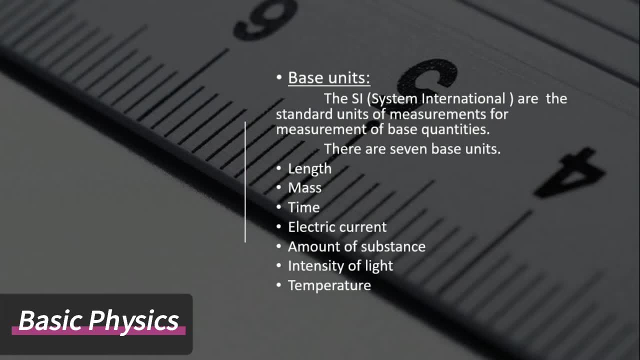 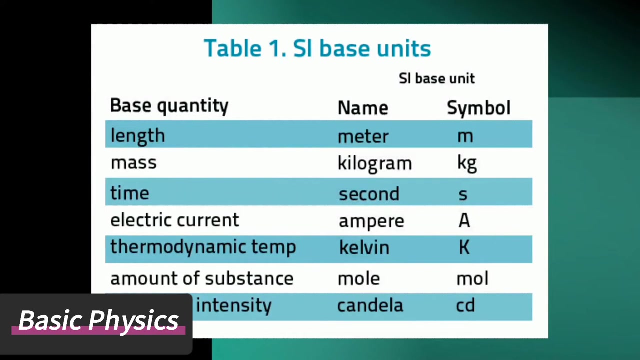 There are seven base units: Length, Mass, Time, Electric current, Amount of substance, Intensity of light, Temperature. Base units are of seven types: Length, Its unit is meter And have symbol M. Mass, its unit is kilogram And its symbol is kilogram Time I. 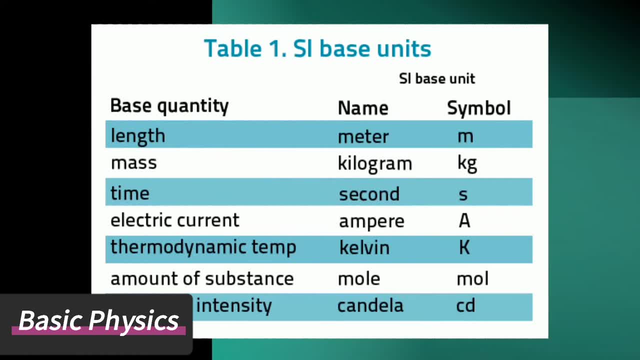 T? s unit is second And its symbol is s. Electric current. Its unit is ampere, And its symbol is a Temperature. Its unit is kelvin And symbol is k. Amount of substance. Its unit is mole And its symbol is mole. Luminous intensity, And its symbol is k. 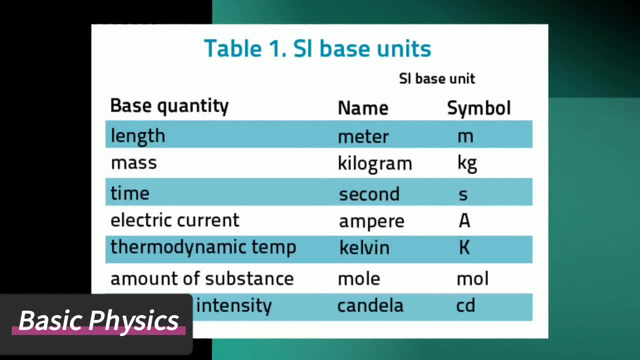 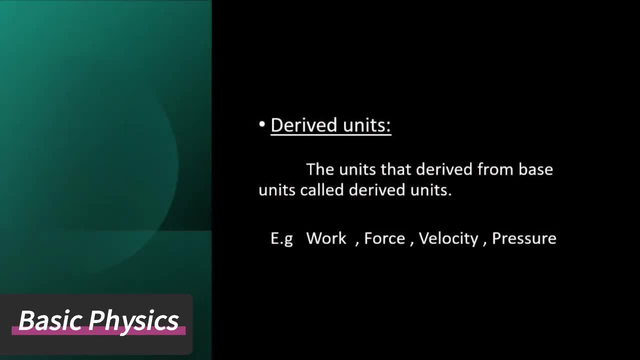 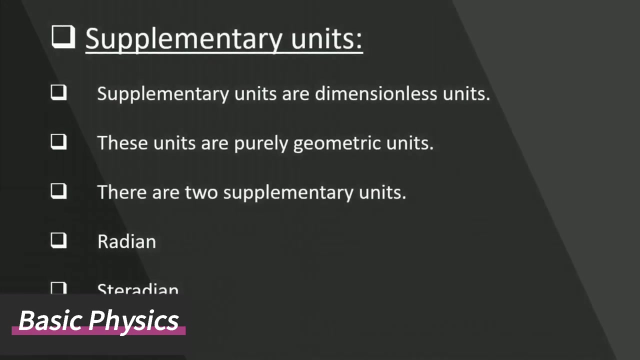 Its unit is candela And symbol is cd. The units that derived from base units are called derived units. For example, work force velocity and pressure Velocity is derived from two base units: displacement and time. There are certain units which is neither base nor derived units. These units are supplementary units. 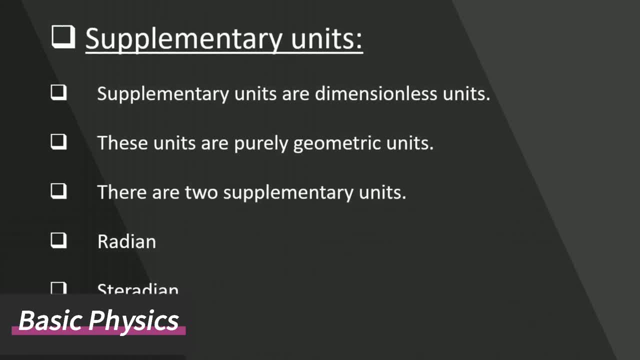 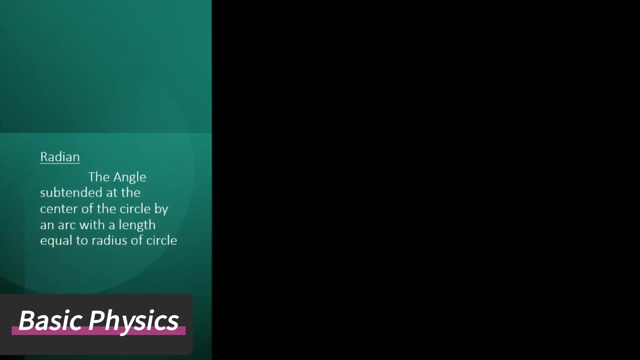 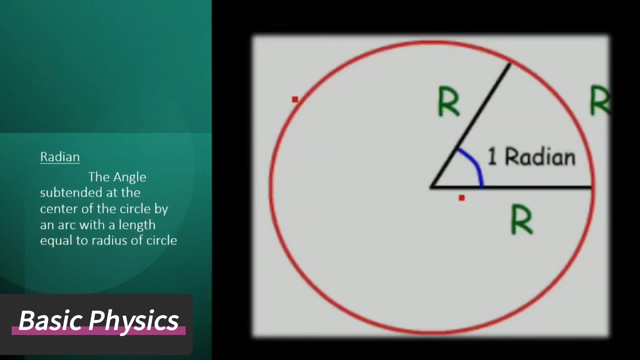 And its symbol is cd. Supplementary units are dimensionists Expressing 전에. These are elements that are based on the홓. Supplementary units are dimensionless units. Their units are purely geometric units. When the arc length become equal to radii of circle, then the angle will be one radian.